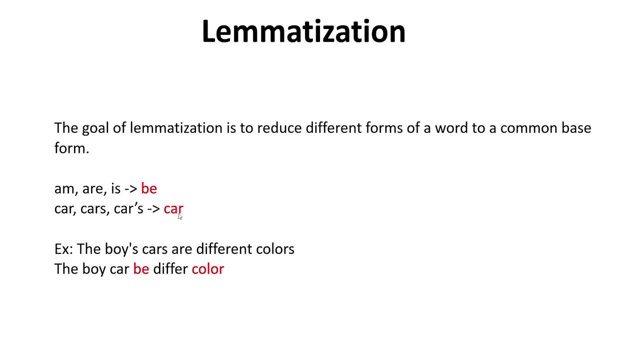 this cars. here, The common base of these words are car. Whenever we will apply the lemmatization, all this word will be reduced to its common base. For example, if you see in your sentence, if you see there is, am, are, is, it will be reduced to be. 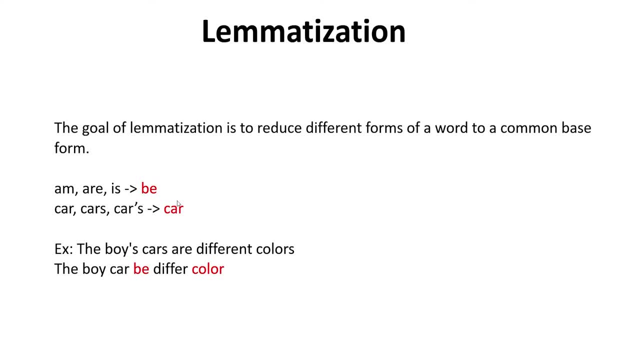 and if you see car cars, cars, it will be reduced to car. And here we have one example: The boys cars are different colors. This is the original example and the. after applying the lemmatization, the example would become something like this: The boy car be. 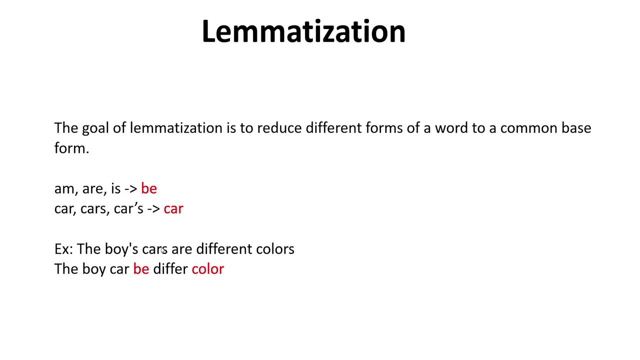 differ color. The form of the, the original form of this words will be the boy car. cars will become car, are will become be and different will become differ and colors will become color. So this is the original sentence and this is the lemmatization. 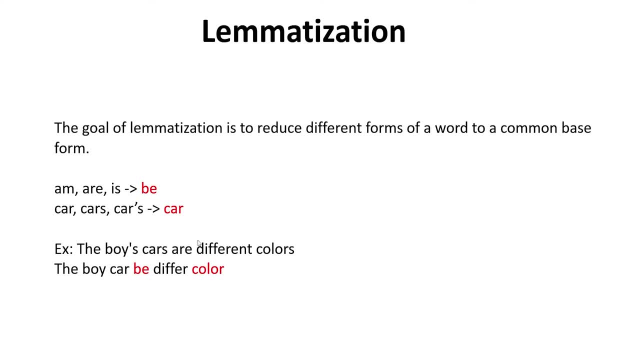 The same here. if you see car cars, cars interisse. these are the Maya. cars are different colors. These are the yellow. your using the C and if you use the green, the colors are at different colors. like losing, You're applying the lemmatization. 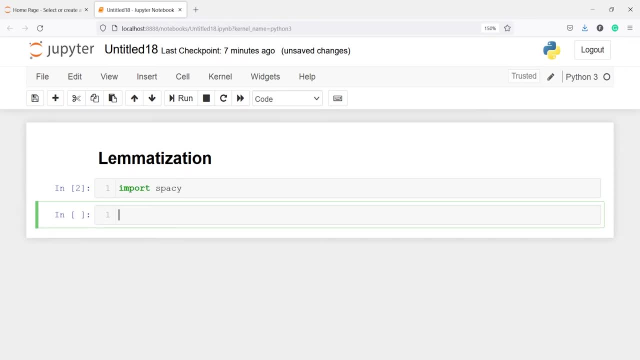 and then this K helps with automating the color of the birds. This is the difference. they come up in the end of the class. These colors work on their self that you're applying the lemmatization: If you use car, you'll use car cars. 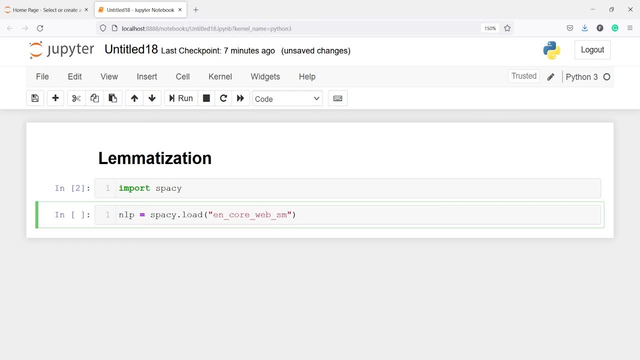 If not, then thejug eight also works hard. If not, then you don't and actually you'll use car. If you don't remap, you can use cars that are not setup for the Lemmatization underscore web. underscore sm. this is the english language model name. let's execute our code now. 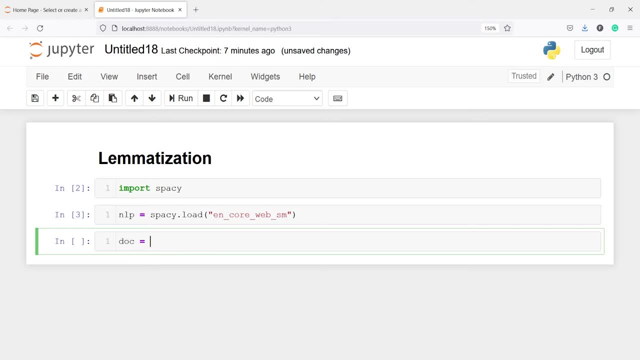 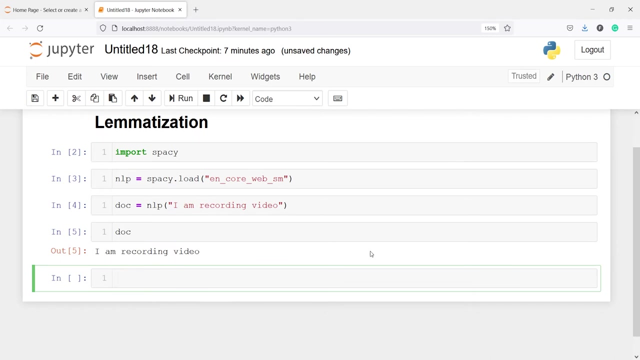 i'll make one variable dog in this. i will save one sentence, i will call this object nlp and then i will write one same statement. let's say i will write: i am recording video, let's execute our code and if i print this object doc, you will see i have this. i am recording video here. 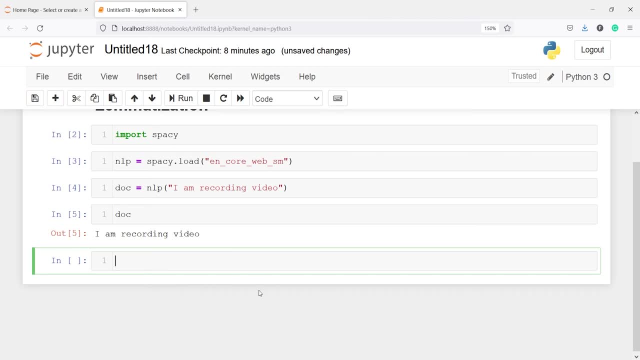 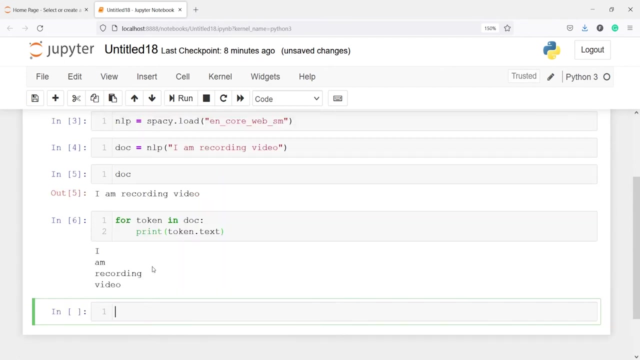 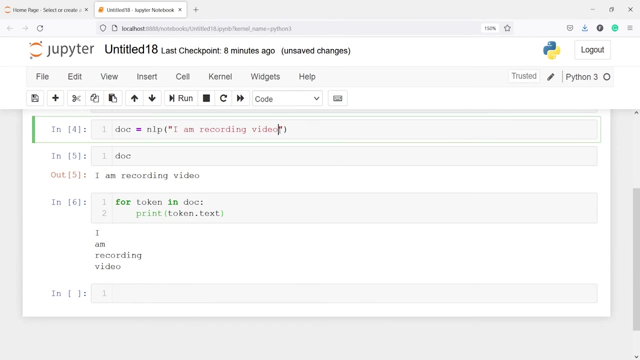 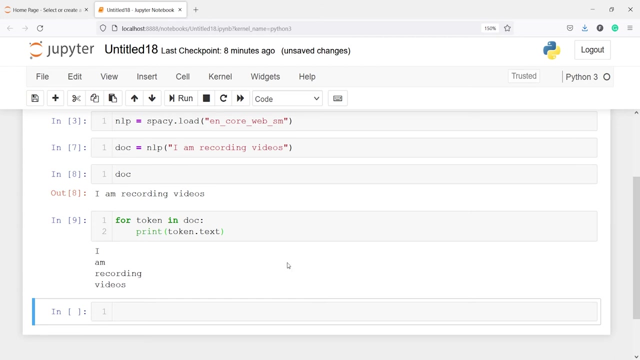 and now let let us tokenize it. i will write for token in document print: token dot text. so we have this text here. i am recording video, or this will be videos, and so we have this. i am recording videos here. now i will limitize it, so this recording. 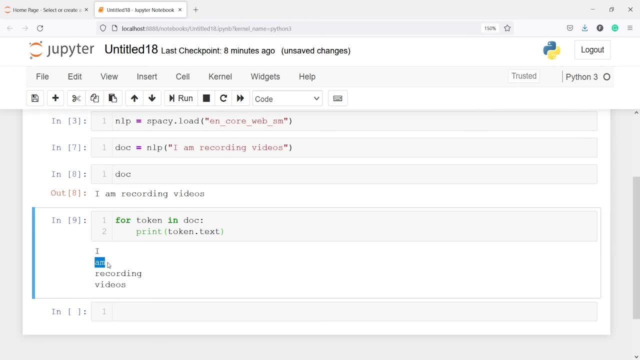 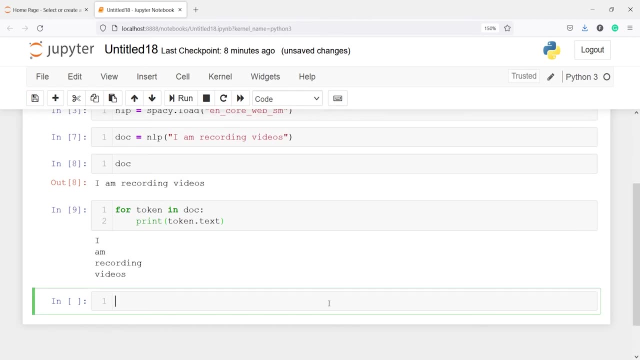 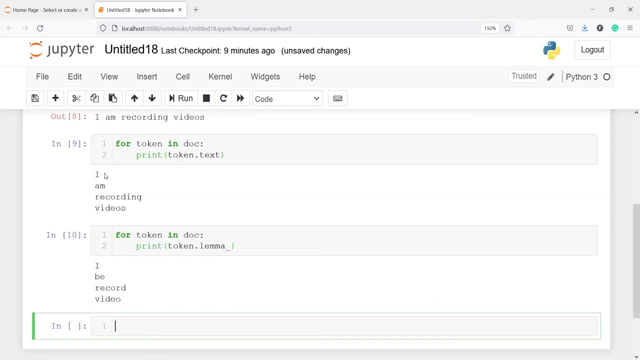 videos. so here m will become b and videos will become video. the s will go, that is, it will come to its root form. and now let us apply that. so i will write another follow for token in doc, print token dot lemma, and let's execute our code. and here in the output you can see this: we have this. 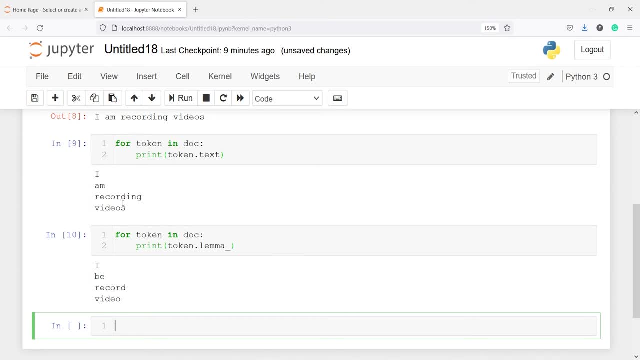 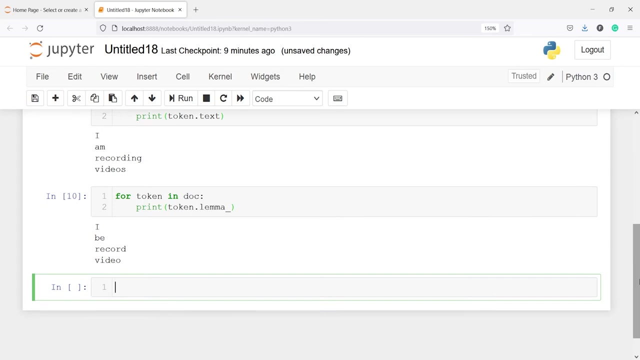 first i, then m got converted to b and from recording it has converted to its base form, record, and then videos has become video. after applying the limitization, all the words came into its root form. let us see one more video example. I'll make one document. I'll make one variable document, doc. then I will. 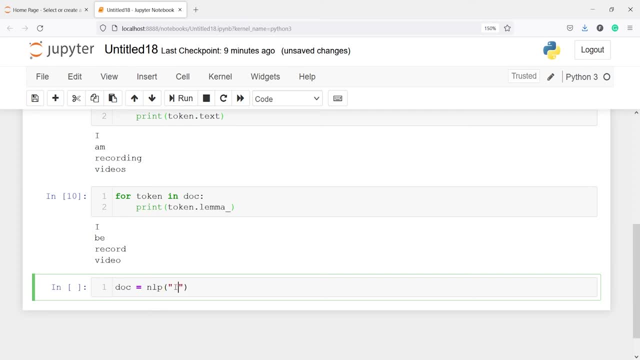 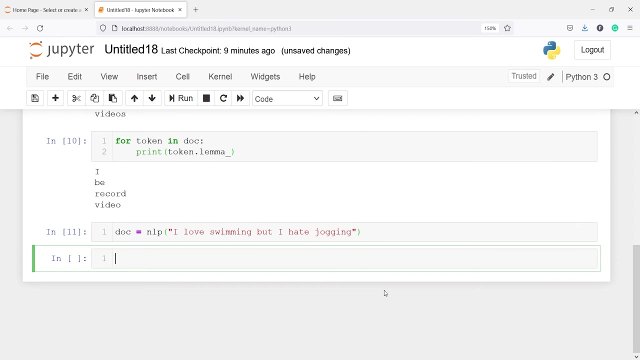 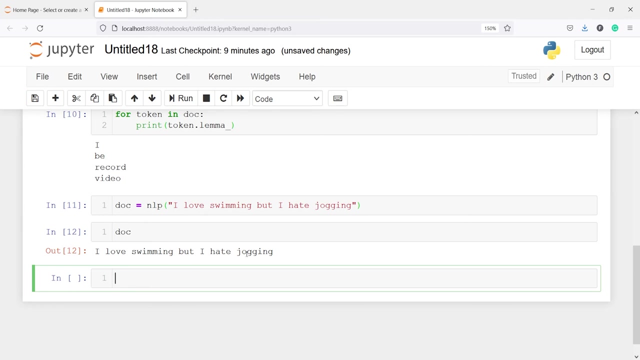 call this object NLP and let me write something: I love swimming, but I hate jogging. this is a random sentence because I don't know swimming, so it's not about me. let us execute our code and if I print a doc, so we have this statement or this sentence: I love swimming, but I hate jogging. now we will. 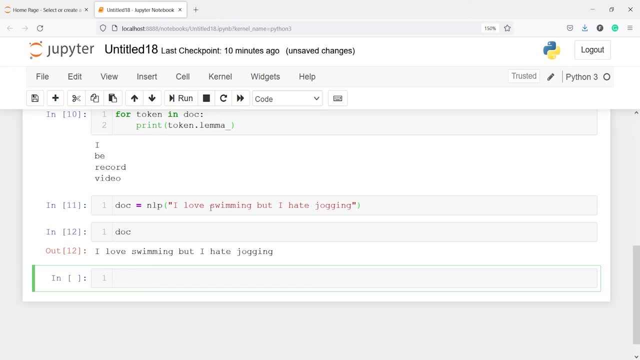 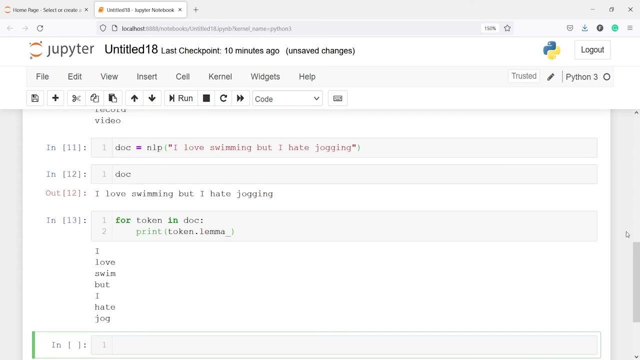 apply this lemmatization and then we will see here swimming will become swim and jogging will become jog. so I'll run a for loop for for token in doc, print, token dot, lemma, underscore, and here in the output again see we have. I love swim, but I hate job. so the 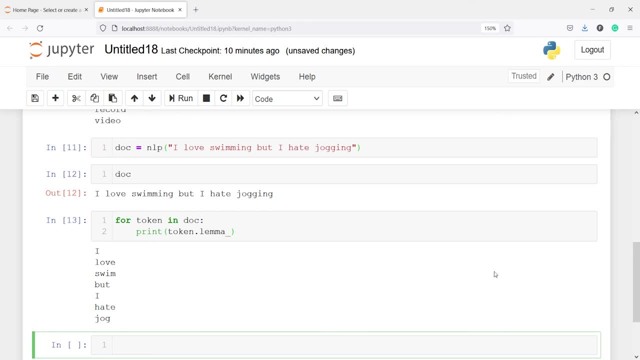 swimming and jogging came to its root form, that- a swim and job. and if you want to get the number behind the lemma that there, then you can just remove the underscore from lemma. so if I remove this underscore and now you will get the numbers there instead of the, so the 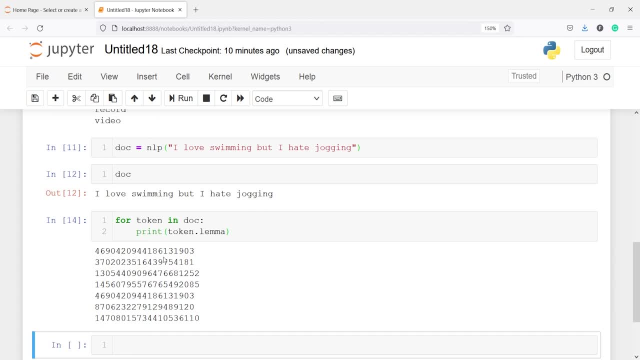 is. these are the numbers. that is the location of the text or the location of the memory where it is stored. so if you remove that underscore, you will get some numbers here. but you always use this underscore here. i was just showing you, but don't use this. always put this underscore and get.